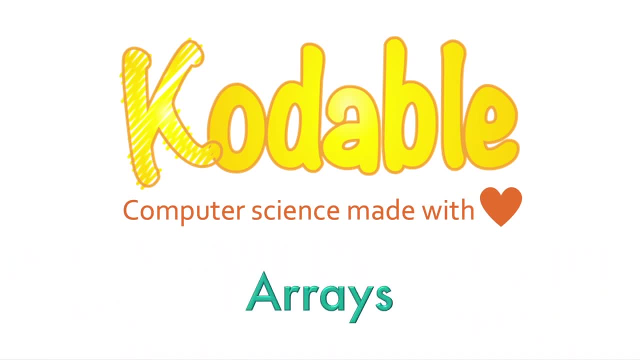 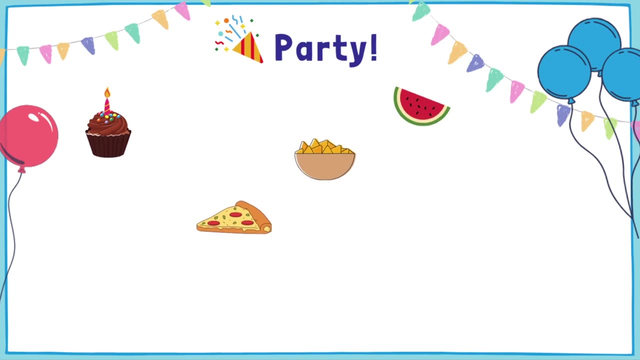 Let's plan a party. There's a lot of stuff that goes into it. You need to decide what food to serve, songs to play and who to invite. When you're planning something like this, how do you keep track of everything you need? You might group all these items into lists. 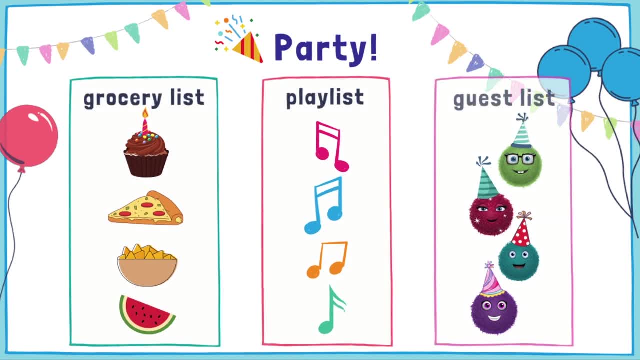 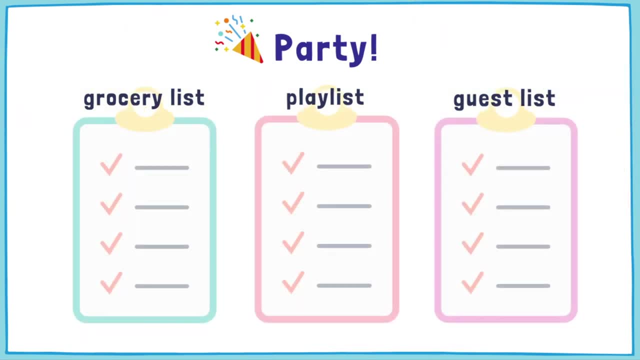 Grocery list, playlist, guest list- All of these lists help you keep related information together and organized. Of course, we use lists every day, not just when we're planning a party. They can help us decide what's most important and think about the big picture. 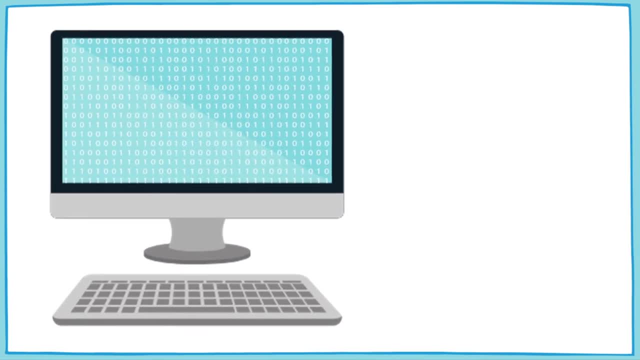 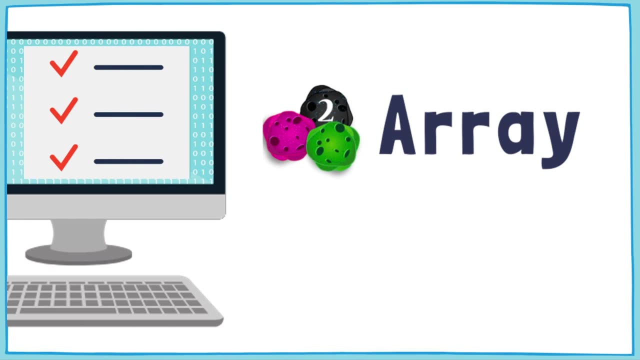 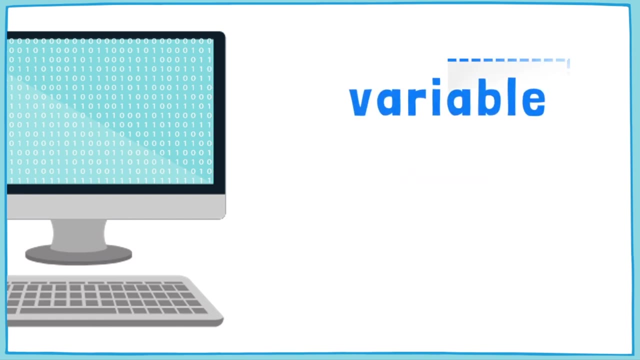 Lists are helpful for keeping code organized too. In JavaScript, a list is called an array. You can store related pieces of data together in one place within a program. So why is this important? Remember, in coding, a variable is used for storing a single value that can change. But as we collect more information, keeping 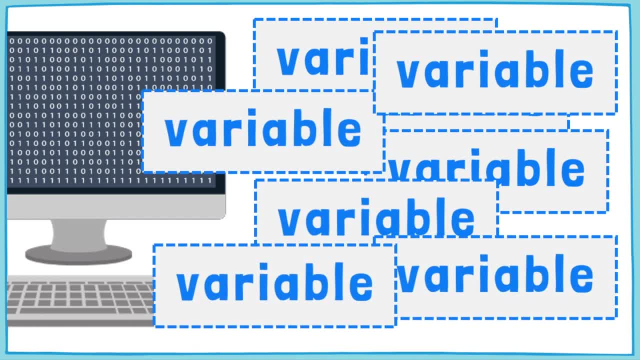 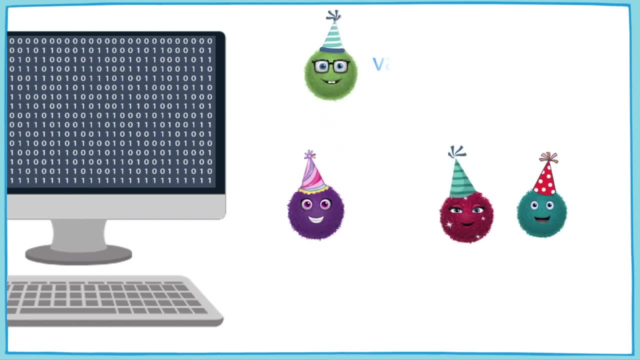 variables organized can be tricky. For example, let's say you want to create a program to keep track of the names of all your party guests. For the first friend, you could create a variable and store their name as a string like this: And for a few names. this is no. 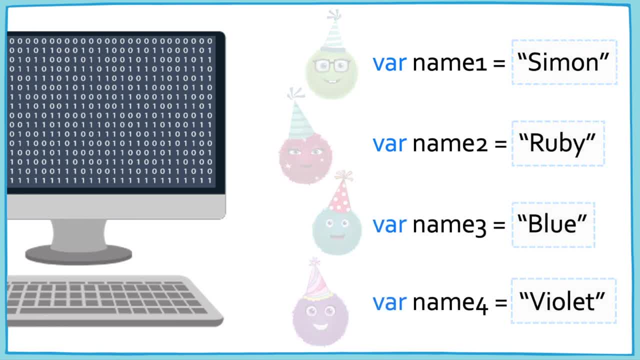 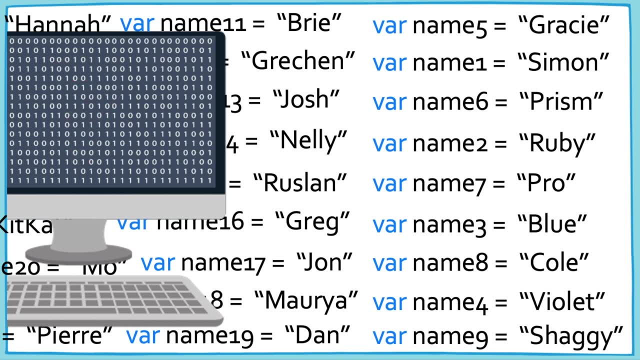 big deal. But what if you wanted to invite everyone in your class Or school? Well, you could do that. Do you even know how many people go to your school? It would be really hard to keep track of so many variables, especially if you don't know the number of names ahead. 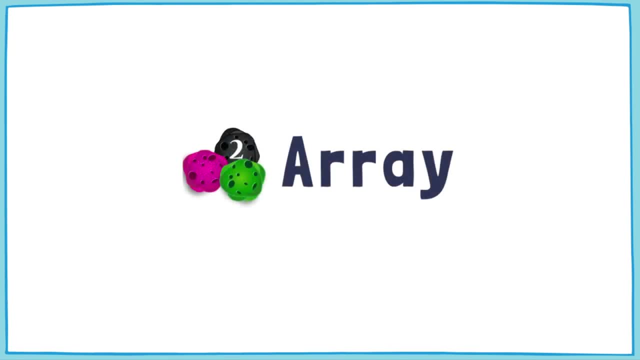 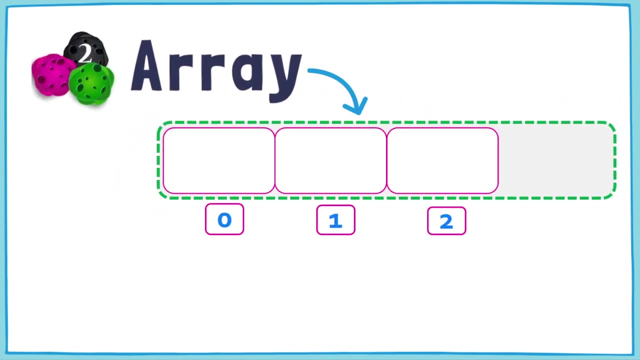 of time. Instead, use an array. An array is like a container that keeps similar things together in a single ordered list. The container can grow or shrink to fit the number of items inside. You might think of an array like a connected row of numbered boxes- Each box 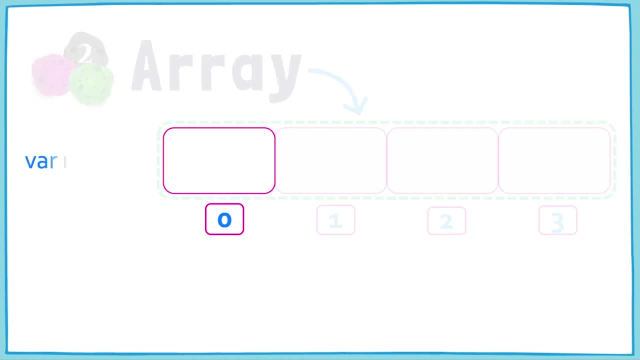 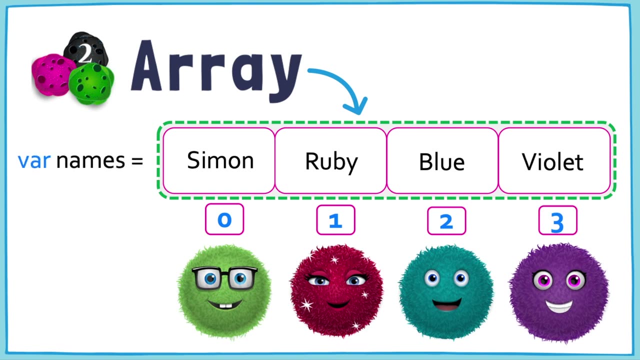 can have one thing in it. Just like you can assign a single value to a variable, you can store an entire array of values in a variable too. This list is only four items long, but in code it could be hundreds or thousands of values. In JavaScript, an array looks like this: Values separated.